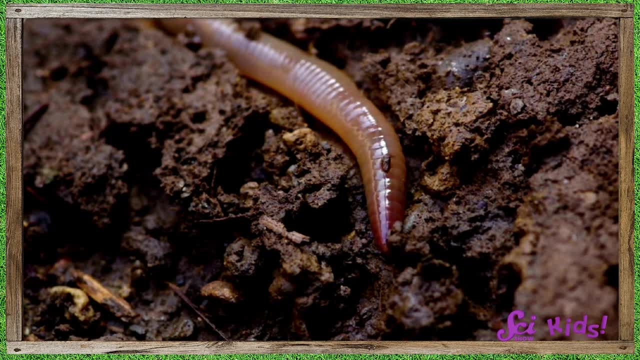 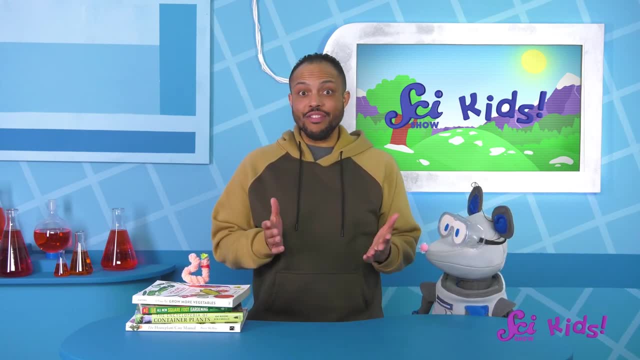 I'm a worm, so I love everything that has to do with soil and dirt. That includes gardening and helping plants to grow from the ground up. We're planning to grow a vegetable garden in this planter box in the backyard, so Squeaks. 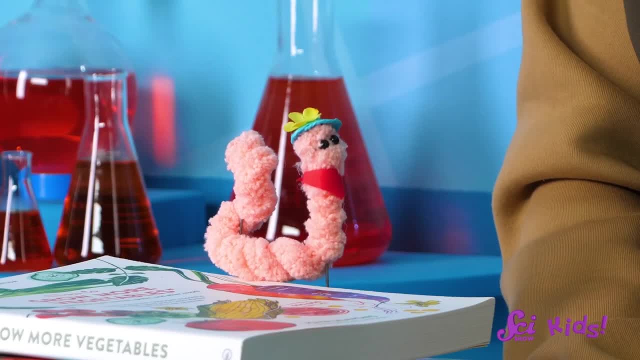 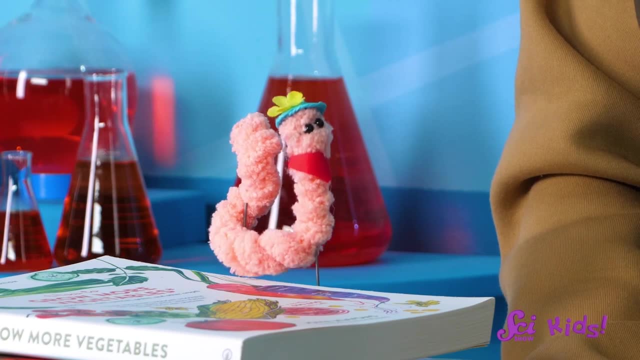 and I can study the plants as they grow this spring. Oh, that's lovely. I'm sure you'll do an excellent job taking care of these plants, but we should also make sure that this space has enough space for our plants. Squeaks has everything you'll need to make plants happy, so they'll grow. 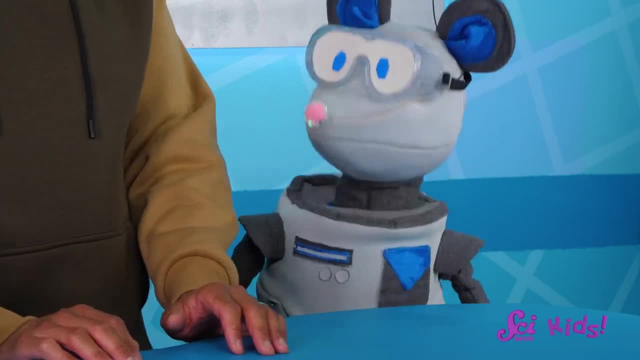 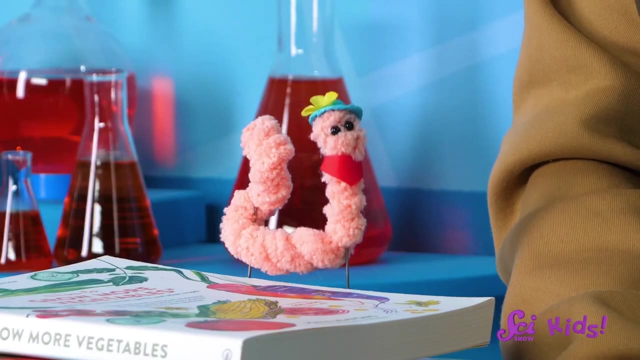 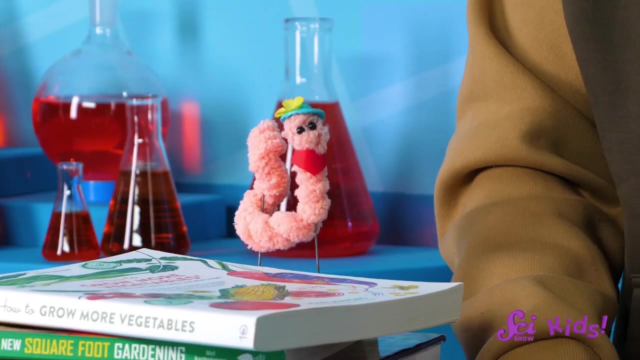 Hmm, what do you think? the plants need Squeaks? Yes, plants need water and sunlight to grow, That's right. And since plants can't move around to find water and sunlight, they also need to be planted in a place that gets enough of those things. 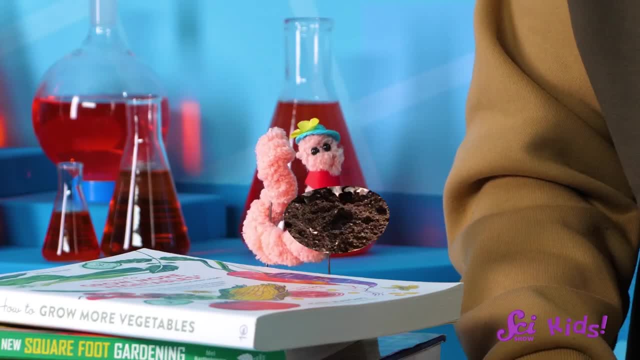 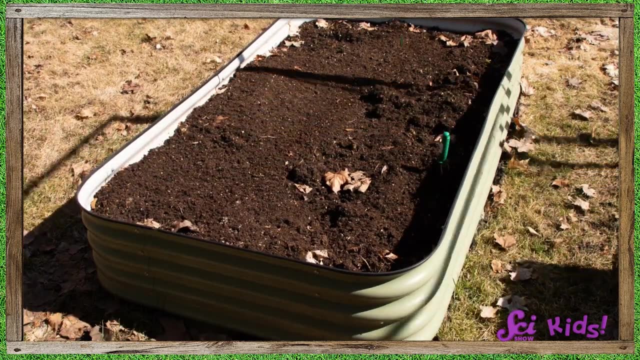 Before you plant anything in it, you'll want to observe your garden bed closely. How much sunlight does it get every day? Is the soil sandy or more like dirt Or even hard like clay? How much water is in the earth here? I sent one of my remote-controlled garden bots out there to help us take a look. 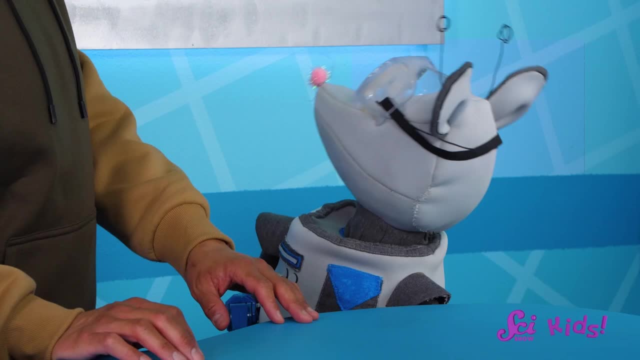 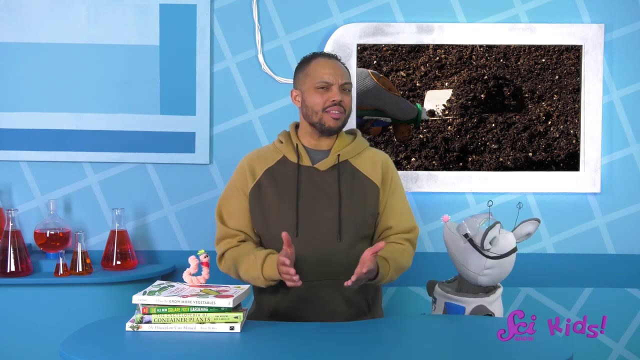 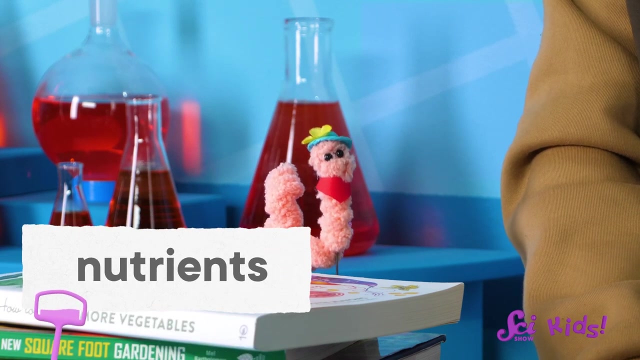 What do you notice? Yeah, the soil is nice and dark and it's not super wet or super dry. I agree This dark soil is full of good nutrients or things that help plants grow, But you may need to water it a bit more once your plants are ready to grow. 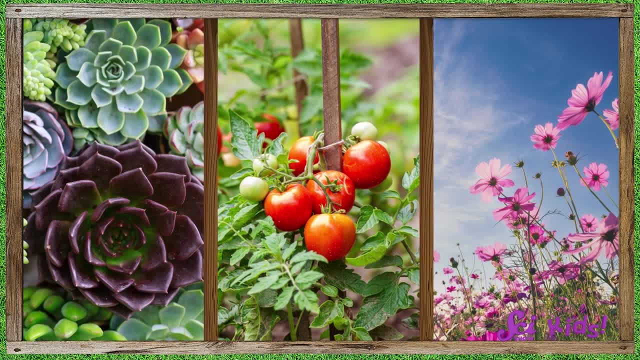 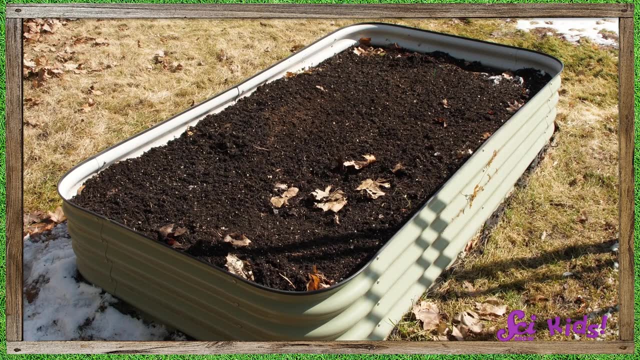 Now, different types of plants all have different needs, and they may need different amounts of water and sunlight. I'm also seeing that there's not much shade here, so you'll want to pick plants that do very well in direct sunlight. The sun will be shining right down on them for a few hours every day. 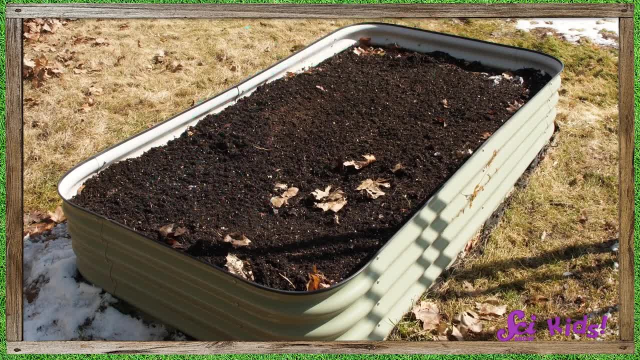 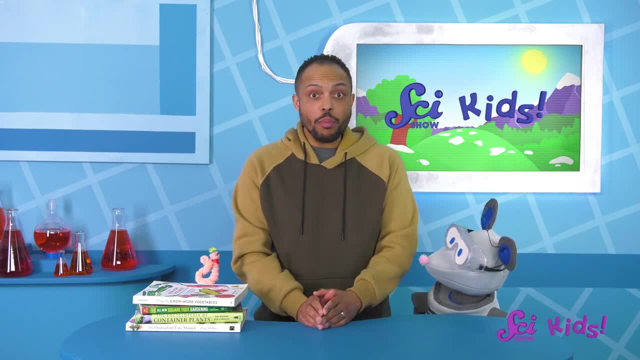 You may need to water your garden on drier days, and you'll still want to pick plants that can handle a bit of rain. Wow, You know so much about gardening. Say, would you like to help us with our new garden project? 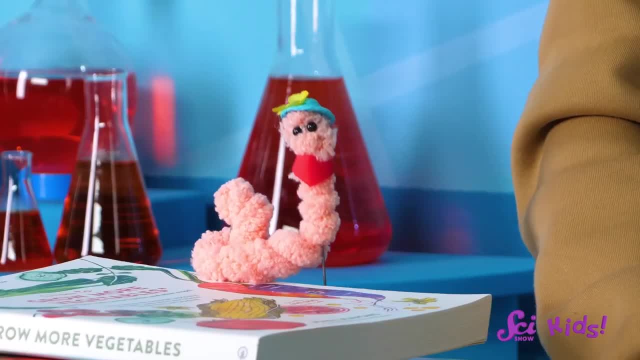 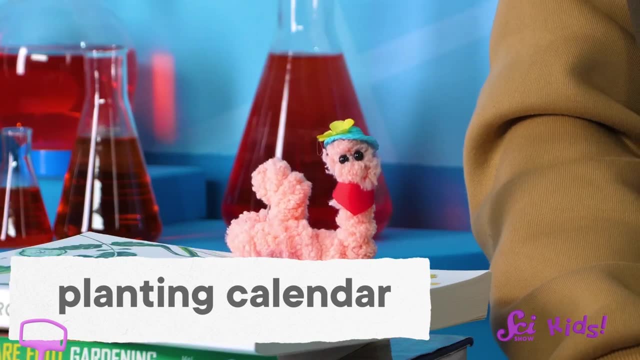 There's still so much we could learn from you about plants. I would absolutely love to help out. Thank you so much for inviting me. How about we meet up soon to create a planting calendar? That's a special tool that will help us to make decisions about our plants.